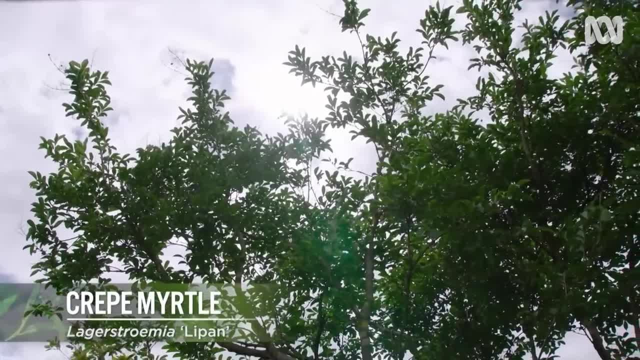 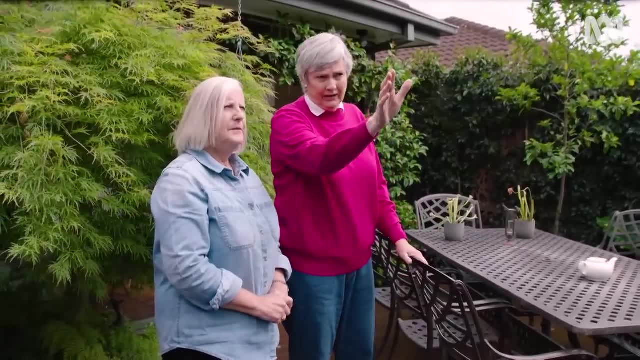 So that's what the crape myrtle is. Yes, the crape myrtle. It loses its leaves, but the camellias that have been freed up and are growing up, they'll cover that space for me And at the back there, the whole way round. 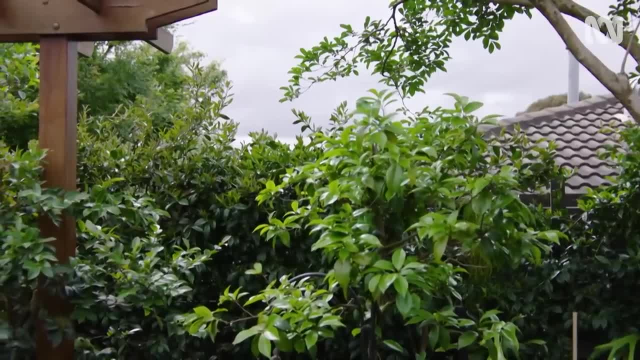 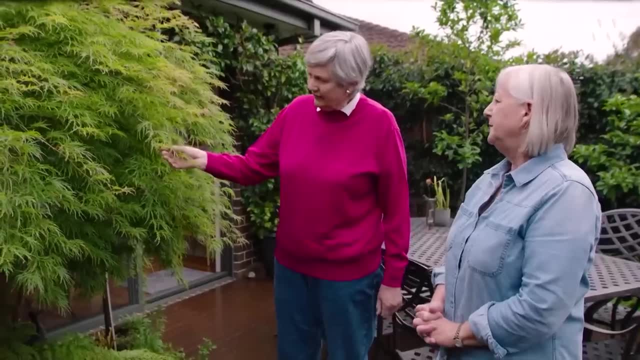 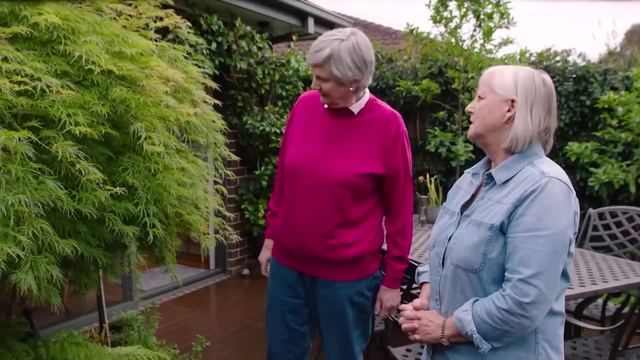 Have you got camellia here? Yes, I wanted a little forest And, of course, this beautiful maple tree. Yes, that's really one of the features. I just love that dissection. It's so beautiful. It's beautiful, It's really. I think it's one of the most attractive Japanese maples, because it's got. 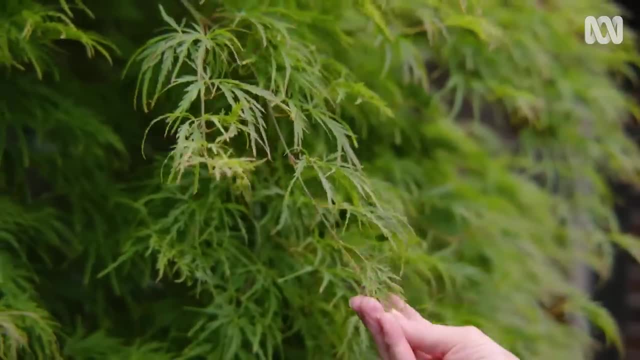 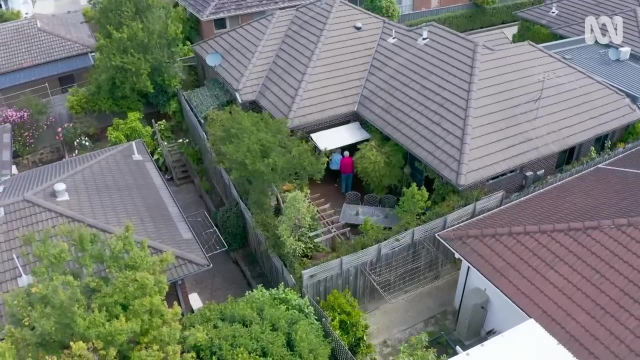 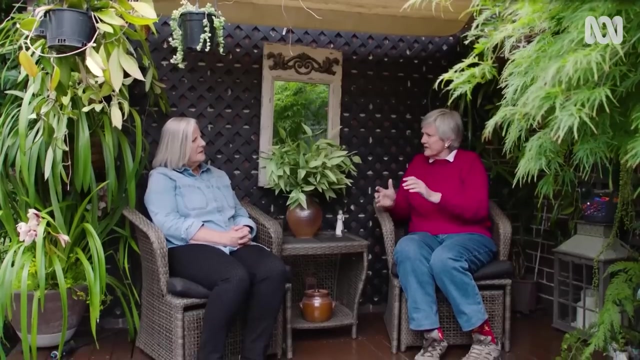 such a lacy, beautiful foliage. It's just gorgeous. This is such a nice little nook and I really think seating is so important in the garden. If you don't have a seat, you're just going to keep working all the time. 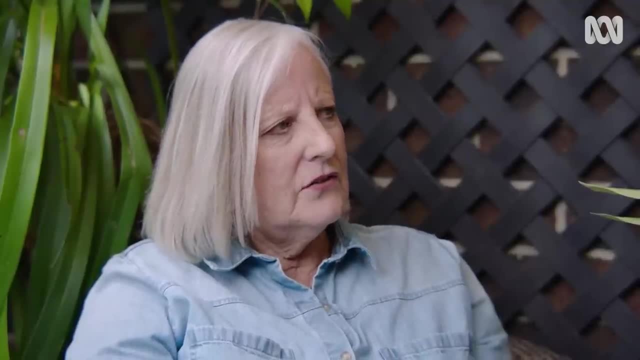 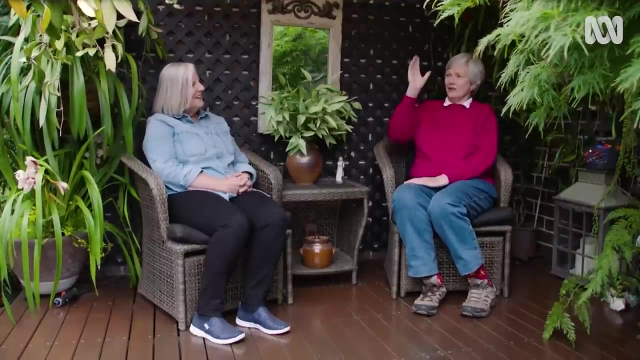 It's absolutely right. We often come out here have a coffee, read a book, just watch the birds. But you've cunningly cunningly created this little area because it's not just a seating area, it's your clothesline. 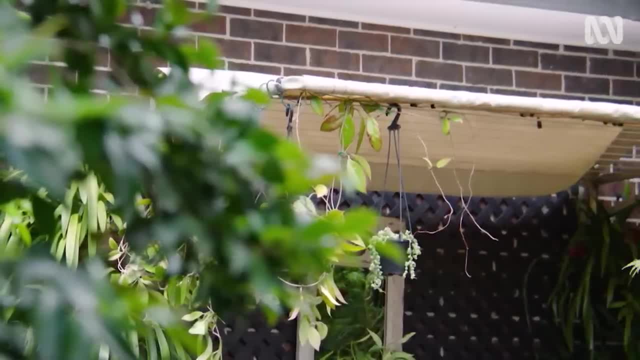 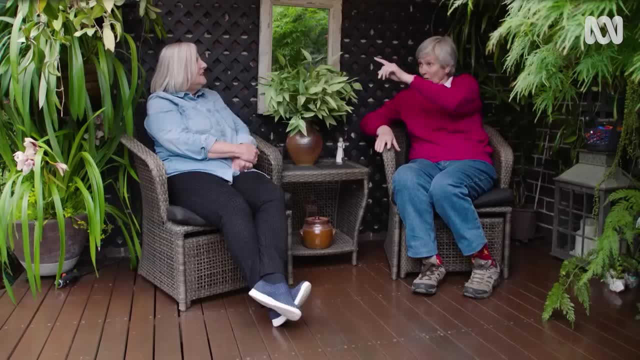 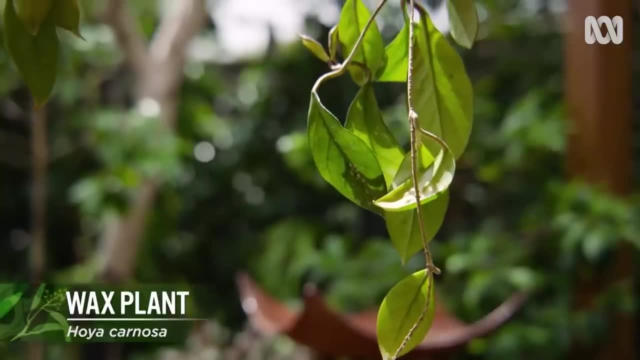 So I thought, well, how do I disguise it? So there's a cover over it, I can still dry my clothes. But also your plants. I like what you've got. You've got the hoyas hanging up. Yes, I've had to use plants which are light in their pots because otherwise I wouldn't want. 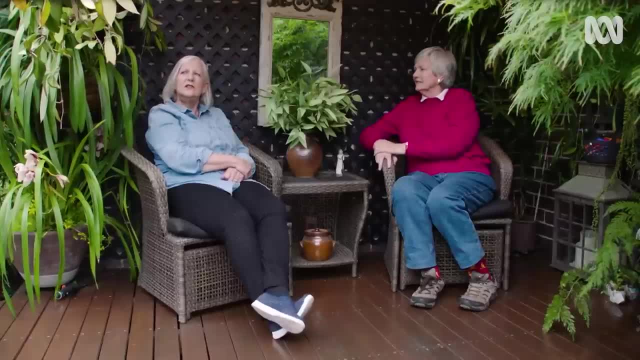 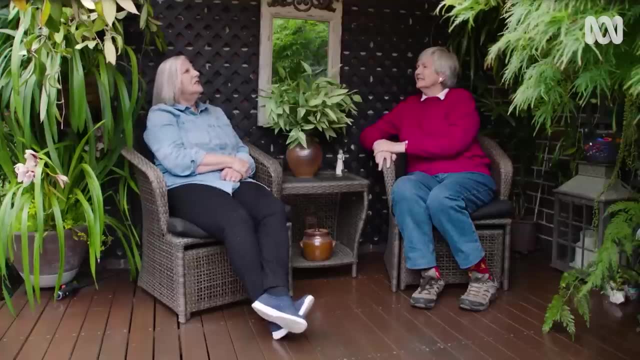 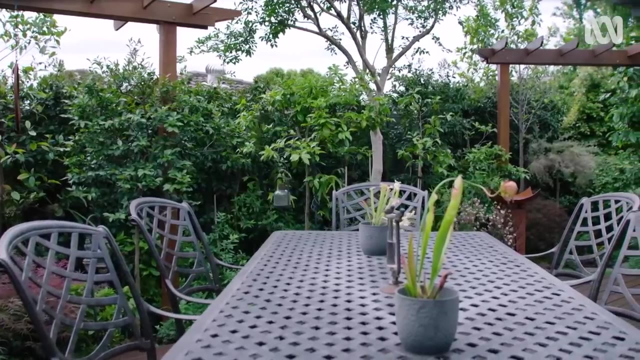 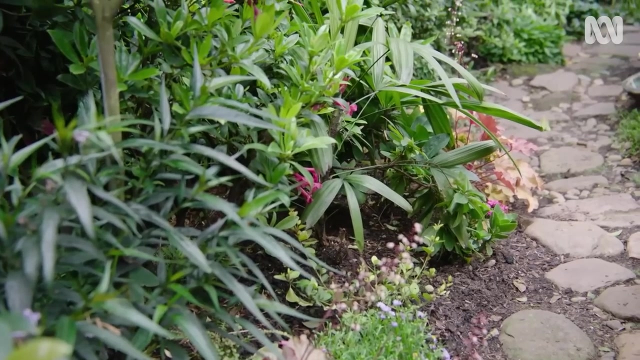 the weight of it pulling down the side of the washing line. So hoya is a good plant for that, And also by using something like that, you can disguise the washing line itself. When you have an almost empty space, it can be hard to know where to start. 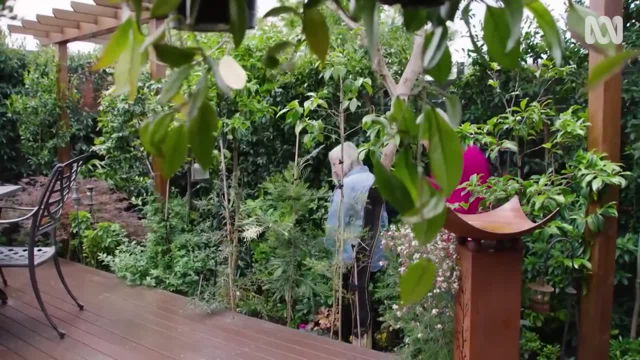 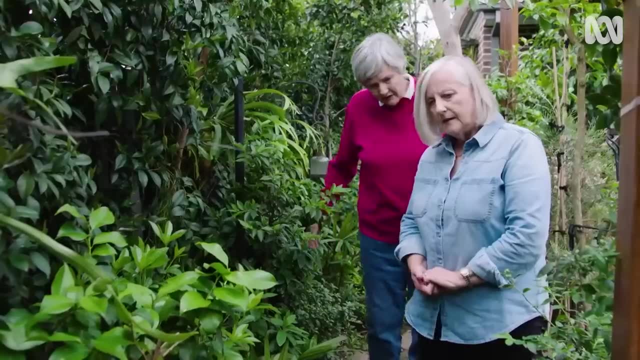 But Jenny went from bland to beautiful by taking her design cues from nature. This is my creek bed. When I first arrived it was a new build, So this little area, tiny though it is, it's got sort of a self-contained feeling to it. 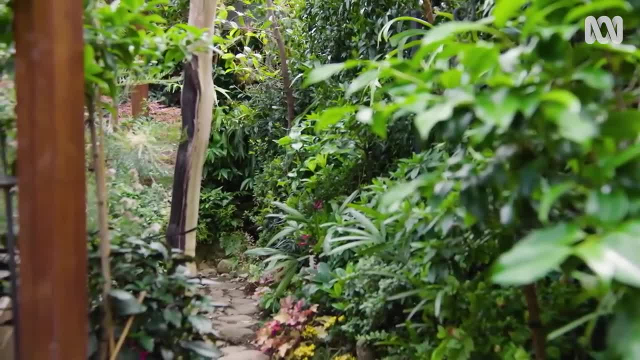 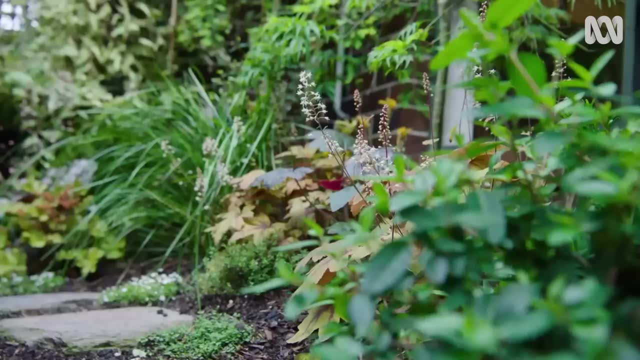 And why have you done it like this, though? I want it to be able to be visible from here, So that you can look down and see the plants and, hopefully, when these grow up- and these grow up- you'll actually be doing a forest walk. 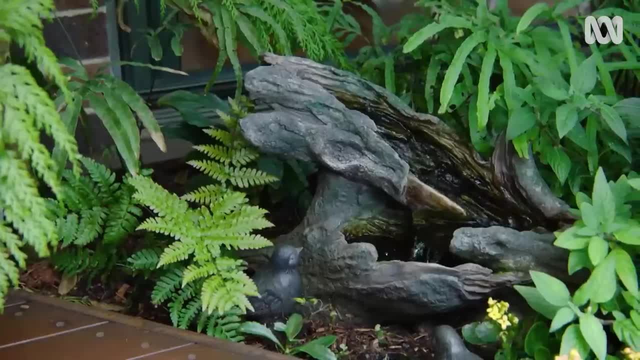 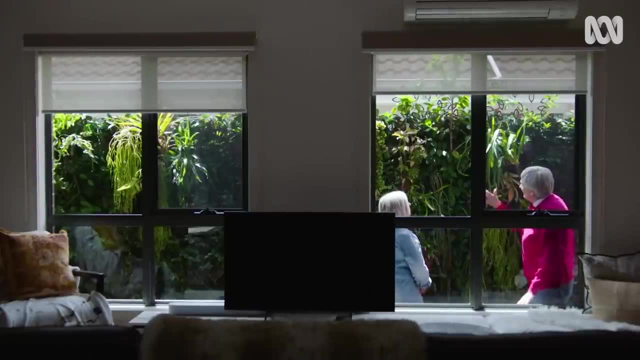 In addition to the main garden area, there are several other small and narrow spaces. One features a wall of epiphytes in pots hanging on a frame on the side fence. This is such a narrow space, isn't it? between house and the fence. 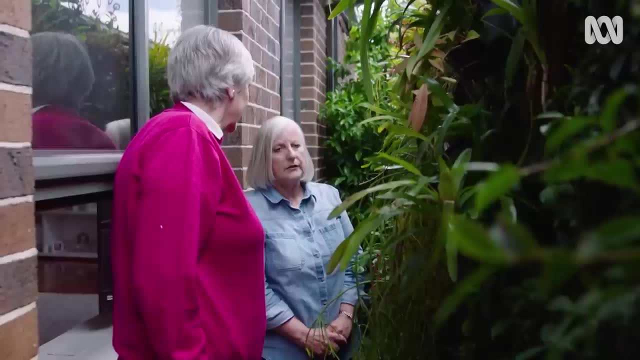 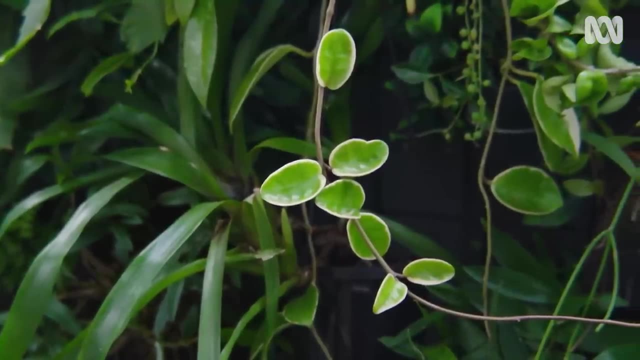 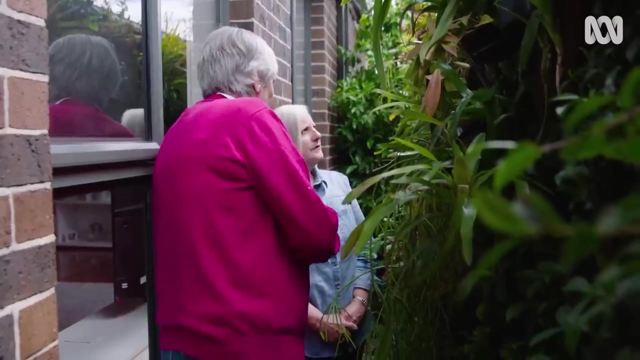 It is, But it shows you can do a lot with plants To cover the wall and to keep your house cool and get variety of planting in as well. It's a whole green wall filled with plants that are literally just hanging in pots And you've got such a lot of variety like this one. 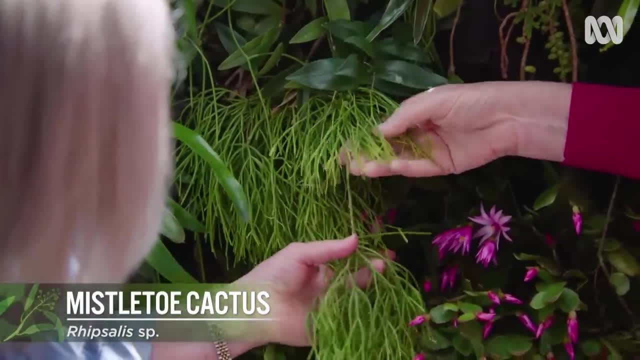 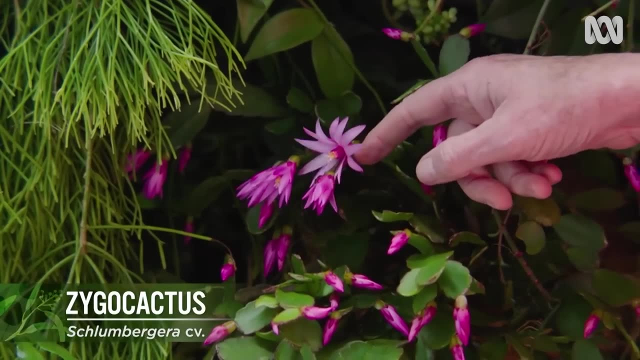 Yes, the ripsalis. It's a great one to have because in a green wall it helps you to blend plants in. I love the zygocactus. The flowers are just beautiful and lovely to watch And it's going to have flowers for ages. 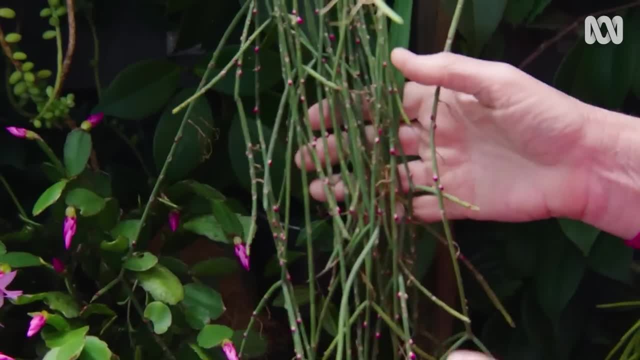 Look at the buds coming on it. Yes, It's a real treat. And this is a treat, Isn't it gorgeous? Oh, another rat's tail ripsalis. It's amazing that they flower. Look at these tiny little things. 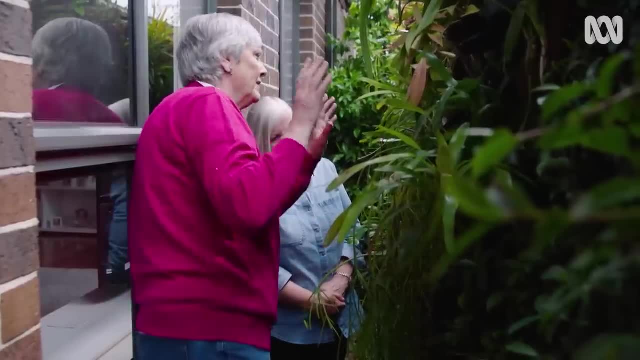 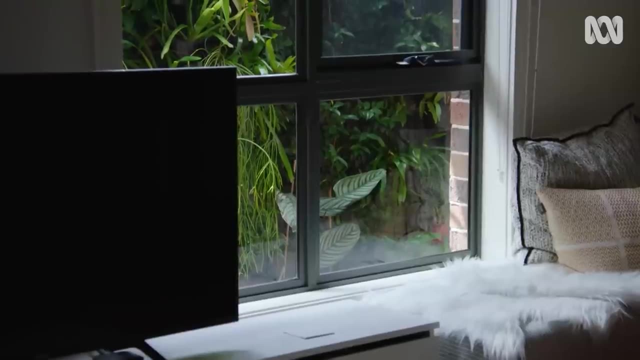 They're just gorgeous. Yeah, that's going to be a mass of flowers. Yes, And all of these are epiphytes. They are, They're just hanging down. It brings the outside in and it's just really relaxing to be able to see this, and it brings. 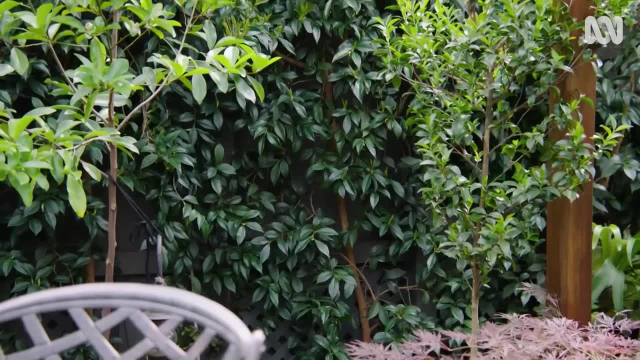 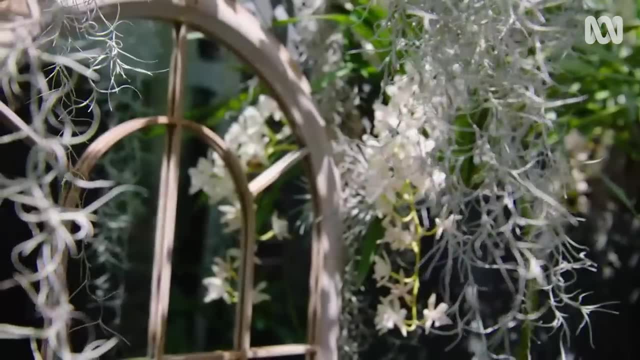 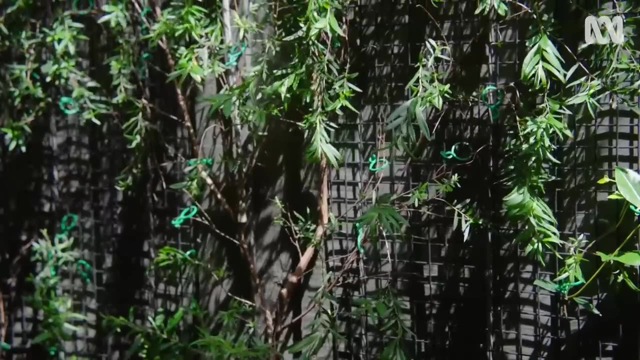 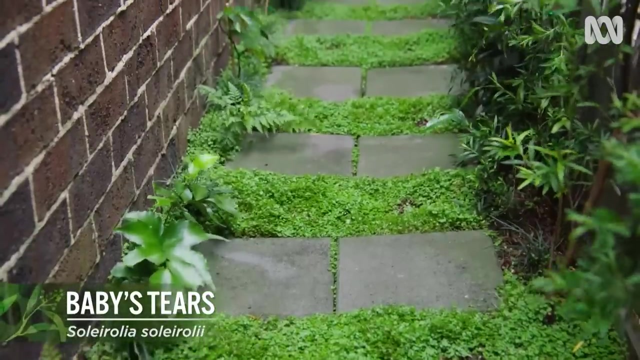 the nature into the house. Another Jenny calls the bayou because of the old man's beard dangling over a seating area On the far side of the unit. Jenny has squeezed even more plants into a very narrow walkway. This baby tears is good in a small area, isn't it? 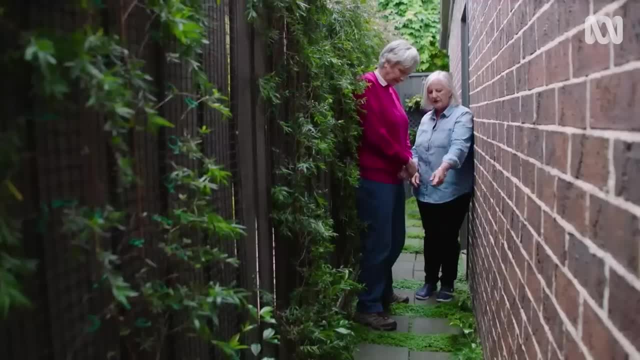 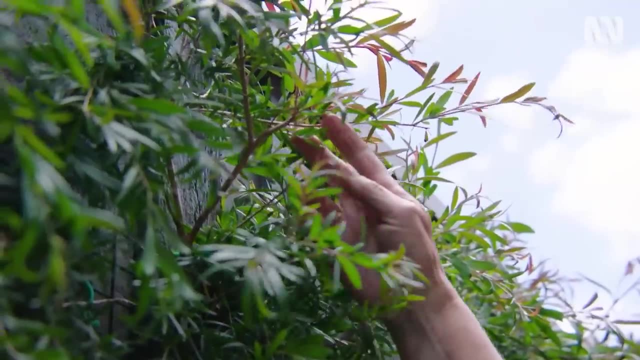 It's great. It just manages itself really. And if you run over the pavers, just pull it off and that's it Done. And this one, this is terrific. You don't often see a tea tree doing that, No. This one's sort of a spaliard along the fence, but I also like to let it run a little bit loose, because it's got a nice weeping habit. Which one is it? That's Leptospermum starinite, And the beauty is you're using the fence again. 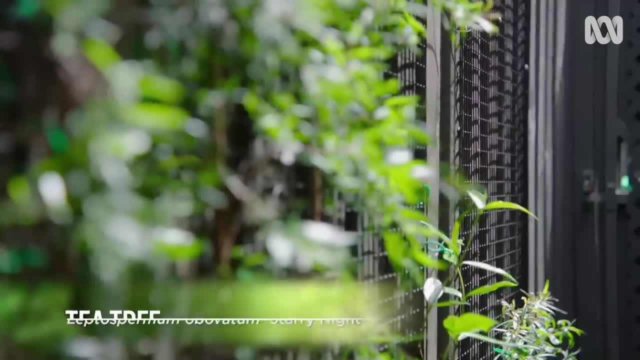 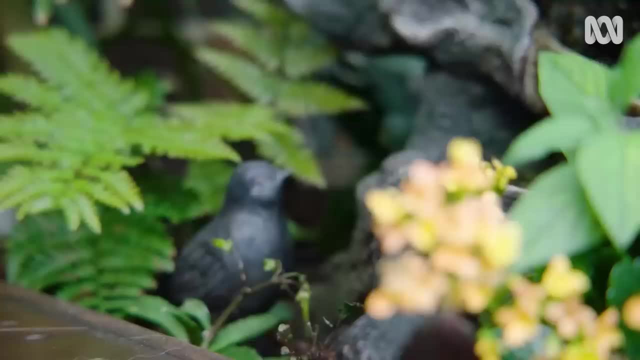 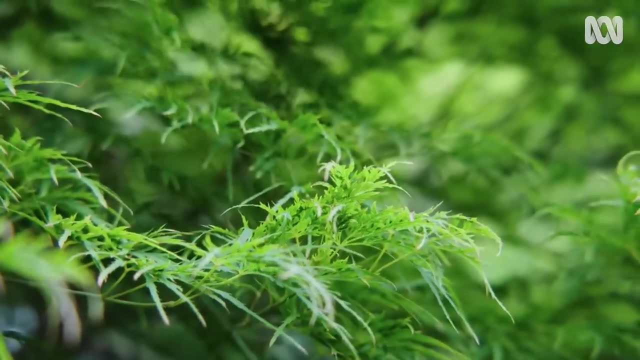 Yes, yes, You have to because it's such a narrow space and you've got to manage the plants in a way that they're probably not growing the way they would. but you can make them do different things. Jenny shows that you don't need to be limited by a small space, but instead you